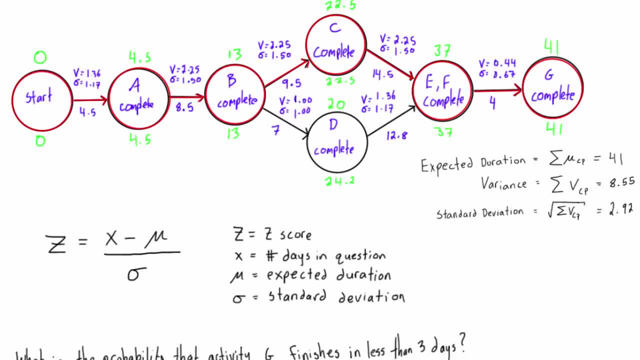 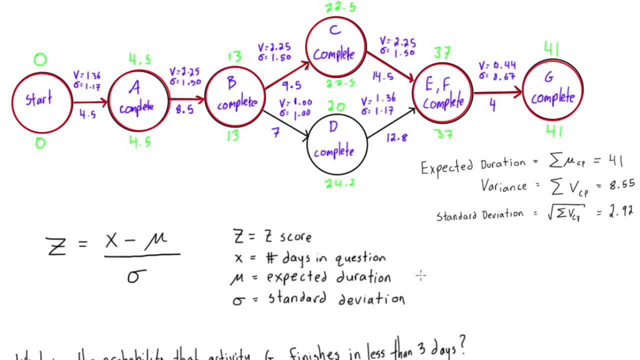 Now we're just going to focus in on one activity here. So let's look at what is the probability that activity G finishes in less than three days. So we know that activity G's expected duration is four days. We can see that here from the network diagram. 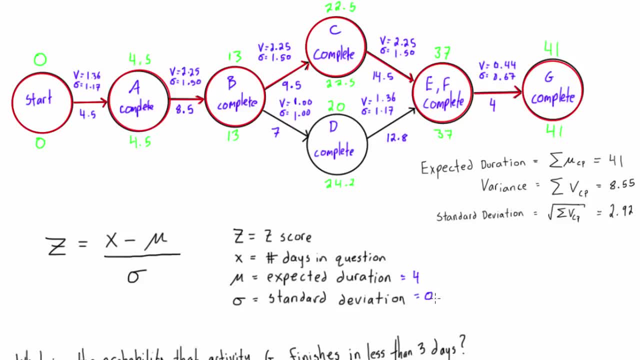 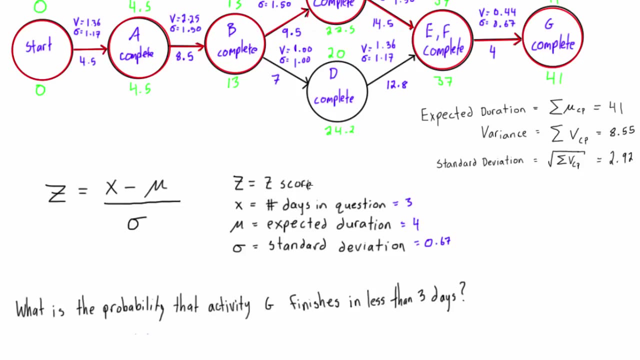 Its standard deviation is 0.67.. 0.67.. And in this case we're looking at the probability that it finishes in less than three days. So for this case, X will be three. Alright, so all we have to do is we just plug in our values into the Z-score equation and we'll use the Z-score to find the probability that this will happen. 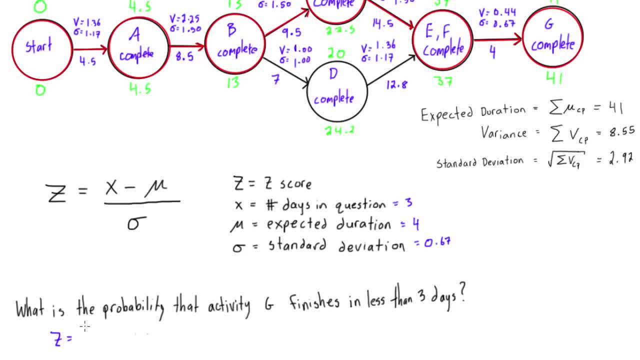 So we have: Z is equal to X minus mu. so we have three minus four, All over 0.67.. Alright, you just punch that in your calculator and you will be getting a value that is negative 1.49.. Just like that. 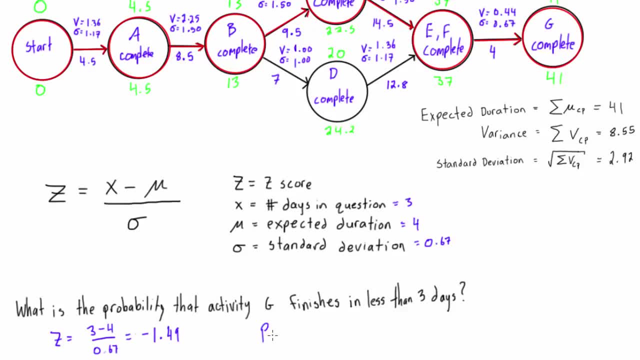 Alright, so then what we do is we take the Z-score. We want to find out what is the probability of this Z-score, So we have to go to the Z-score table for that. Let's put in some arrows. Alright, so we go to the Z-score table. 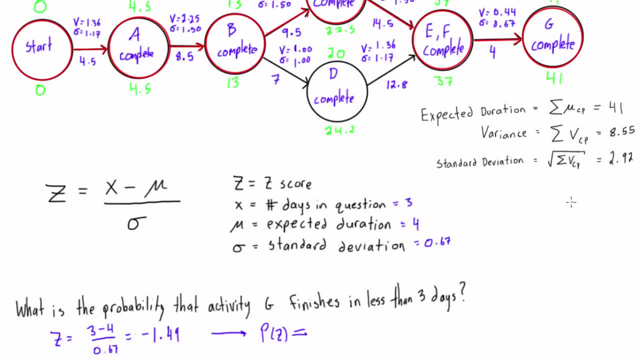 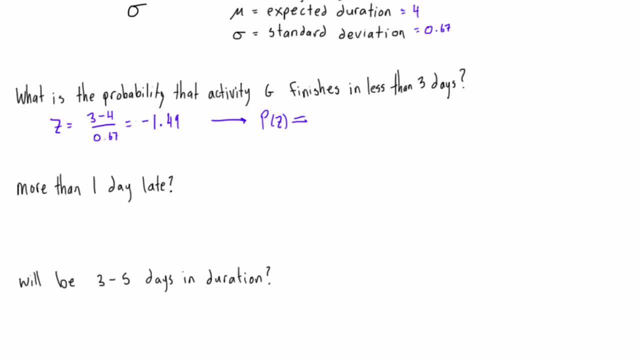 Again. you can find it in any statistics book or just Google image searches Z-score, Z-score tables- you'll come up with a ton of tables, so I just found one down here. We are looking for the probability of the Z-score for negative: 1.49.. 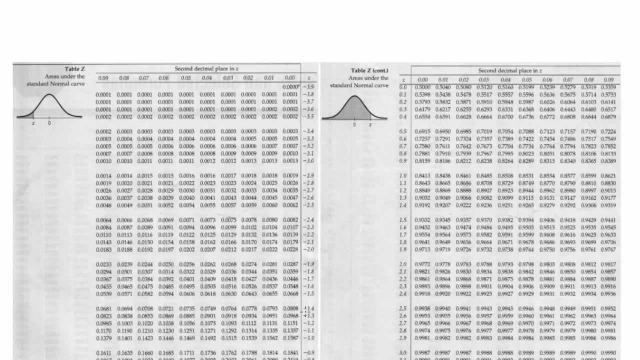 So, if you remember from the last video what we do, we find negative 1.4 and then 0.9.. So if you combine these, we would get negative 1.49, which is the Z-score that we have. 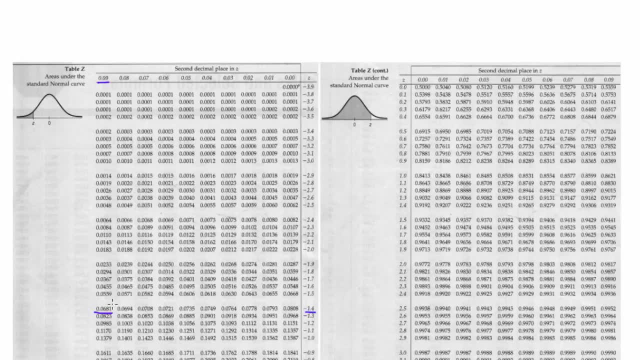 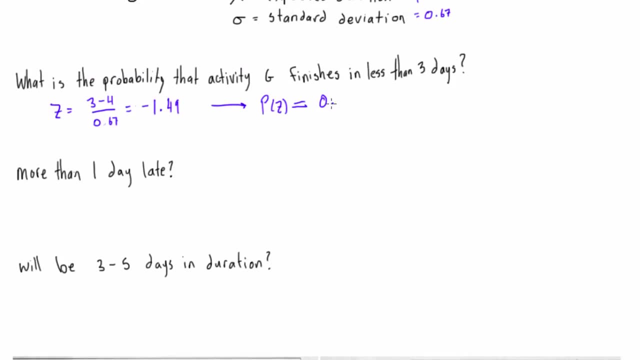 And you see where these meet up And we get. the probability is giving us here is 0.0681.. So first of all, let's write that down: So 0.0681.. But what does that mean? We need to make sure that we're actually getting the right value here. 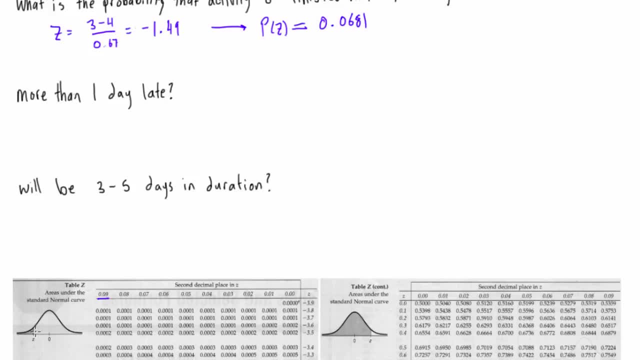 Well, that's saying the Z-score tables always give you the probability of landing in the shaded area. So if you consider this central part of the bell curve here as our mean, our mean was 4. And X we were using was 3.. 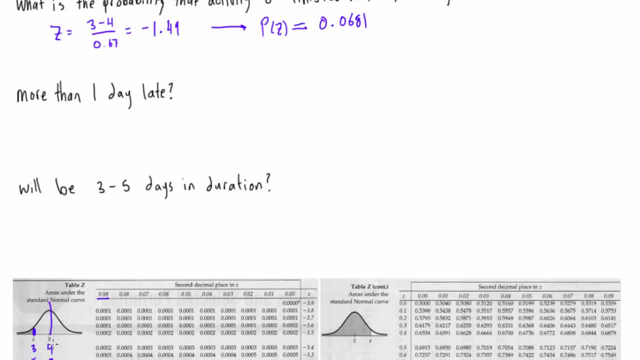 So let's even label that We have mu and X. So, given that mu and that X, we have this standard normal. Well, that's the standard normal, But we're translating it to be our just a normal curve, Because now it's centered at 4 instead of 0.. 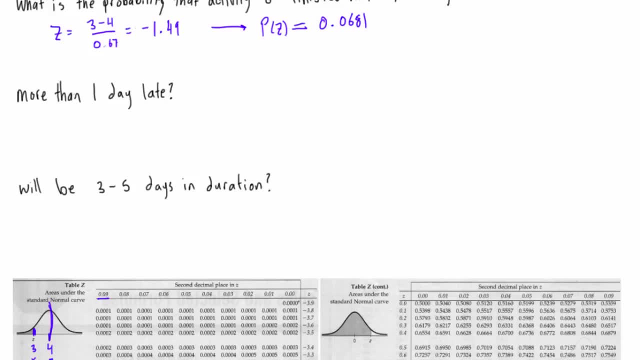 So there we go, Just like that, All right. So what this is saying is: this is the probability that we'll land in the shaded area, And that's the probability That's 0.6.. So that's 6.81%. 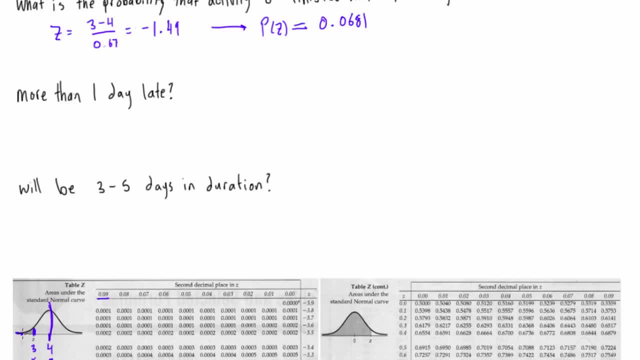 You just multiply that by 100%, So we have a 6.81% chance of landing in the shaded area down here, And that is the area that is less than 3.. So that includes 2.5 days and 2 days and 1 day and so on. 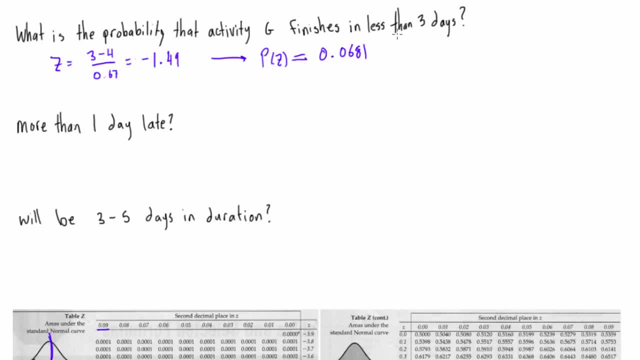 So if that's what we're looking for in our question- the probability that activity finishes in less than 3 days- then yeah, that's exactly what we're looking for. So then we can say that our probability that is just 6.81% chance. 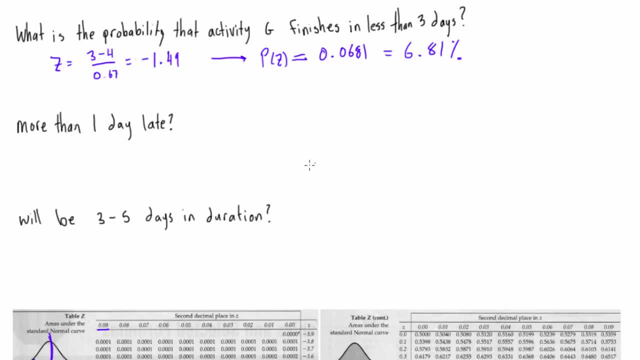 that this activity finishes in less than 3 days, All right. So now let's look at the alternative. Let's say what if it's more than 1 day late? So we have our Z score again, We're not. our X won't be 1 here. 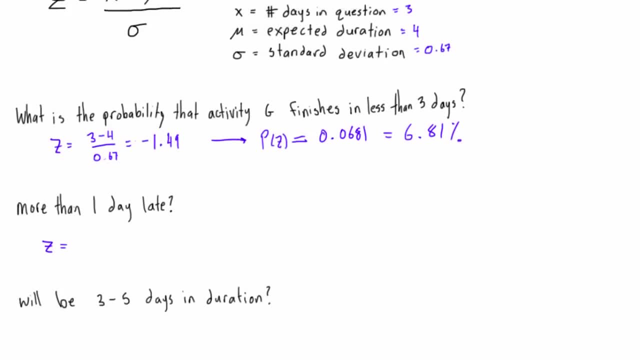 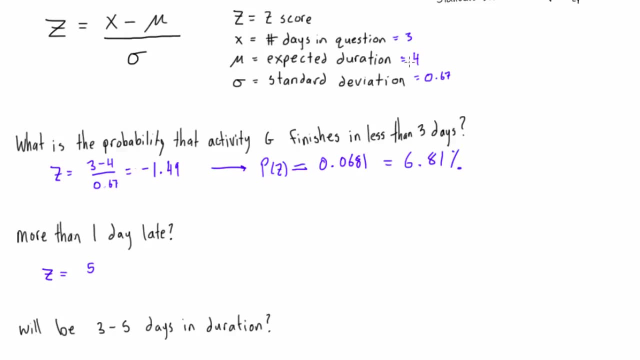 This is more than 1 day late, So we're knowing that our our expected duration is 4.. Then this would mean our X would actually be 5 in this case, right, It would be 4 plus 5.. Okay. 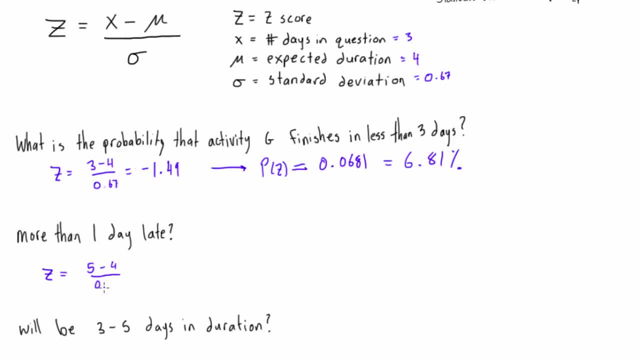 So we have 5 minus 4 over 0.67.. All right, So 5 minus 4 over 0.67.. That's just going to give us the same but positive, So that'll be 1.49.. All right. 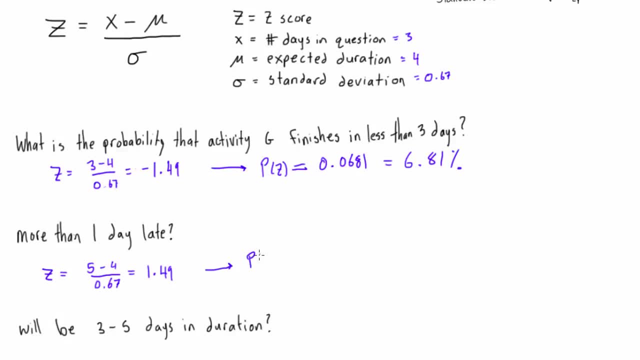 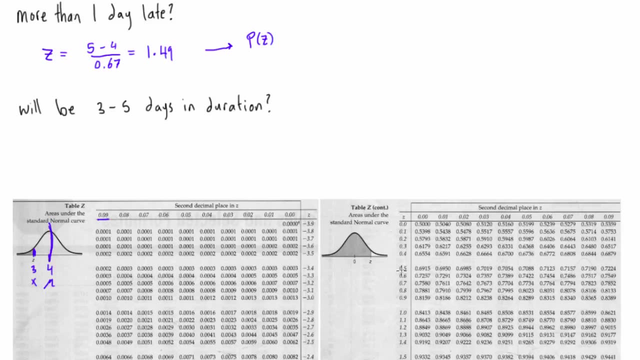 So now we need to look up the probability of this Z score and figure out what that even means to us. So we come down here. We're not even the negative Zs anymore, So we need the positive. So we have to locate 1.4, which looks like it's right here. 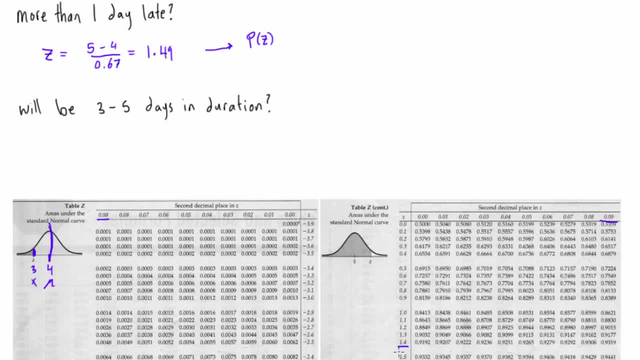 1.409.. Combine those You get positive 1.49.. And then we see where they intersect And it's giving us this value here. So first of all let's write that down. That is 0.9319.. 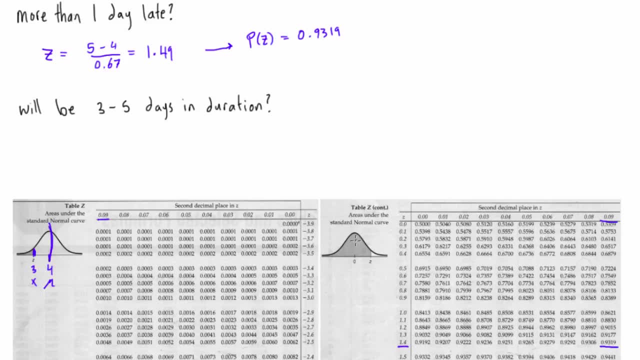 9, 3, 1, 9.. Okay, So again, let's just figure out what's even going on here. We're not using the standard normal curve, We're using the just normal curve, So it's not actually centric. 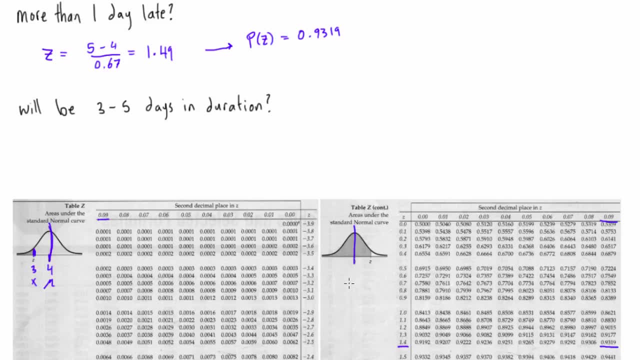 It's centric at 0.. What the mean will be in our case is 4.. That's our expected duration for this activity X. in our case. we've said this is 5. And that's also. you're seeing, it's one day longer, right. 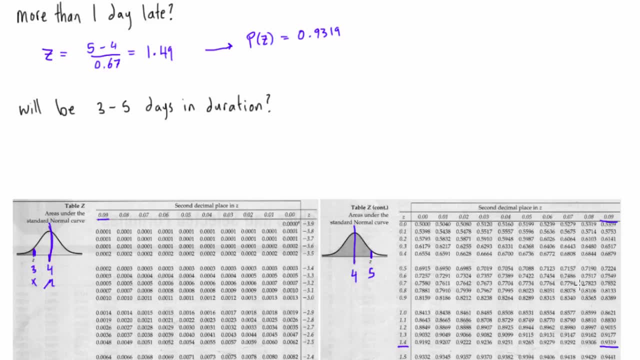 More than one day late. So this is actually returning This Z score. the probability of this Z score returns the possibility of landing in a shaded area. So what it's saying? if you multiply this by 100%, there's a 93.19% chance that the project will finish. 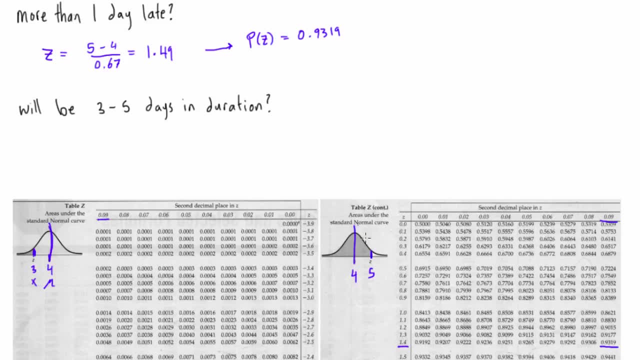 in less than five days. But we need, we need the probability that it will finish in more than five days. So what we do is we have to subtract 1 minus this. We have 1 minus 0.9319.. And the reason we do that? because the 100%. 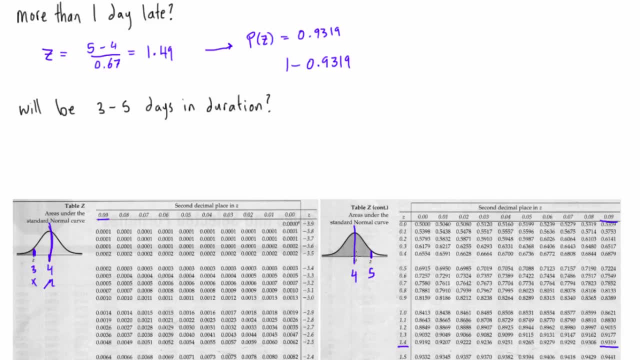 of the possibilities lie under the curve. So you can also think of that in terms of unity or 1.. So if the whole area under the curve is 1, then the shaded area would be 0.9319 or 93. So we're looking at. 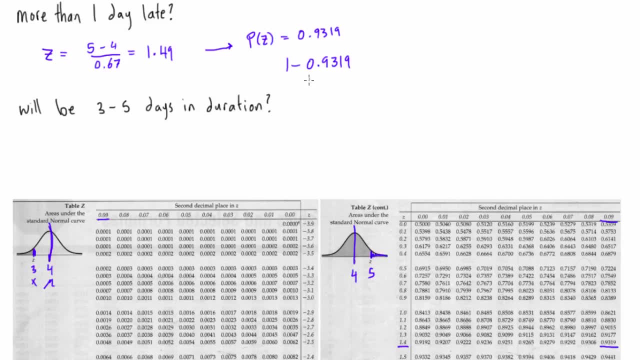 This area here, actually, which would be blue. So it's just 100% minus 93% or 1 minus 0.93, however you want to look at it, And when you subtract that, you'll actually see that you get 6.81%. 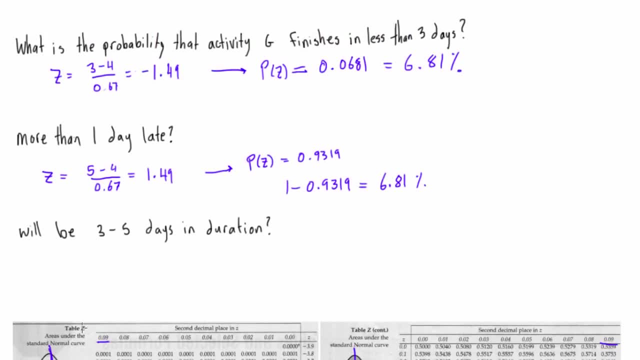 And that's interesting because if you come up here, that's what we also got for the probability of being less than three days, It's the same as being more than one day, like more than five days, And that's because they're both one day away. 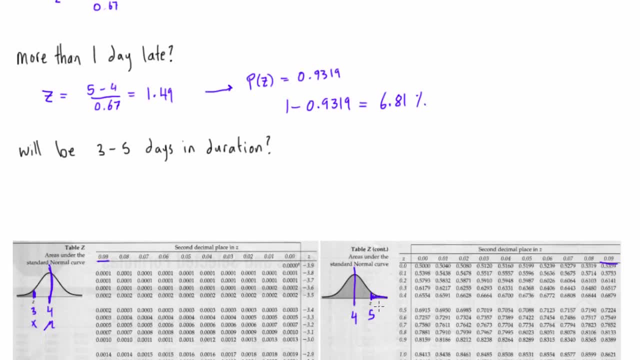 by looking here, Three is one day less than four and five is one day more than five. So you're actually seeing that, yeah, the probability of being more than one day late is 6.81% and the probability of being less than one day early. 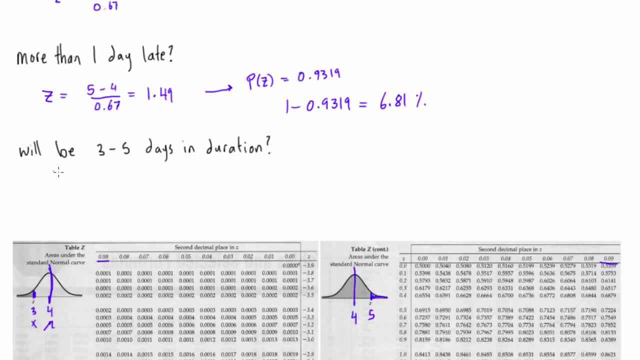 or more than one day early, I suppose, is also the same. So that brings up the question: is then, what is the probability that we land between three and five days in duration for this activity? Well, let's draw ourselves a little bell curve here. 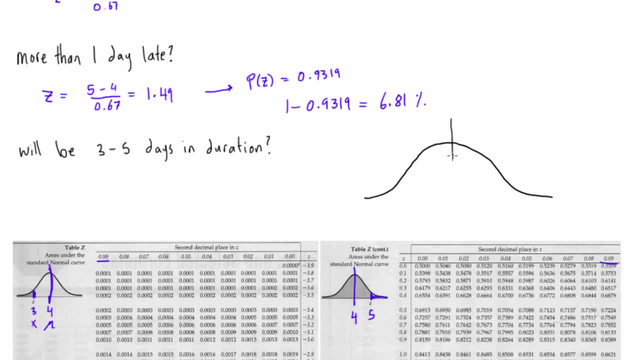 So It's not as good as the ones in the diagrams right below, but it'll get the point across, All right. So let's label this We have here. let's actually clean that up a little bit. Perfect, All right.